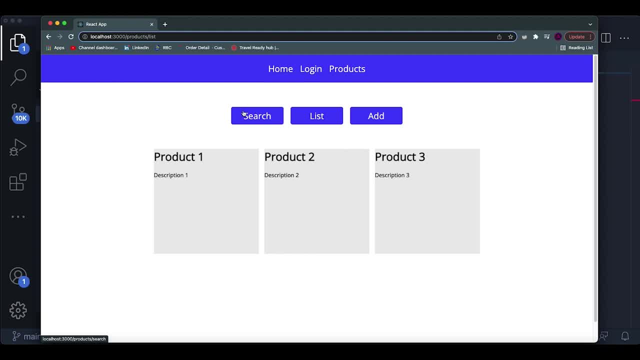 creating nested routes a lot easier and a lot cleaner, in my opinion. Now, in order to explain exactly what nested routes are and how to implement them in your project, I created this little demo over here, which is just a simple website. If you want to check out the code for it, it's going to. 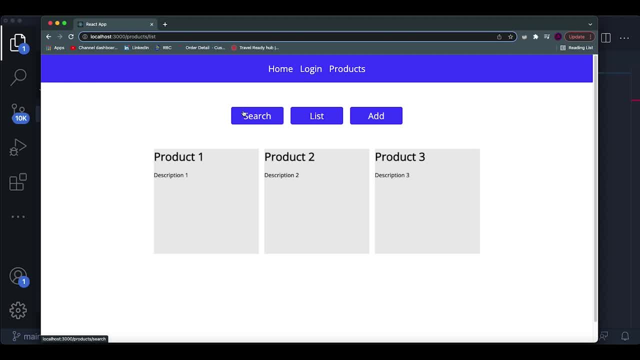 be in the description, together with the code that we write for this tutorial. But basically, imagine you have a website where you have a navbar right And you have multiple routes, for example, the inside of it. there's multiple different things you want to display, For example, in the products. 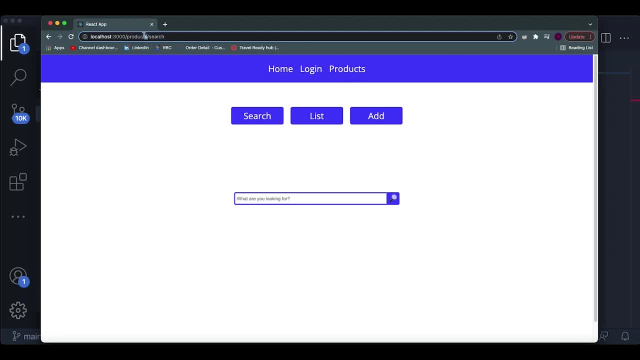 page we have all the products routes, but then inside of the products route we have other routes, such as the search routes, where you see the page displays this little search bar. Then there's the list page which basically just display like lists of products. Maybe you can add a. 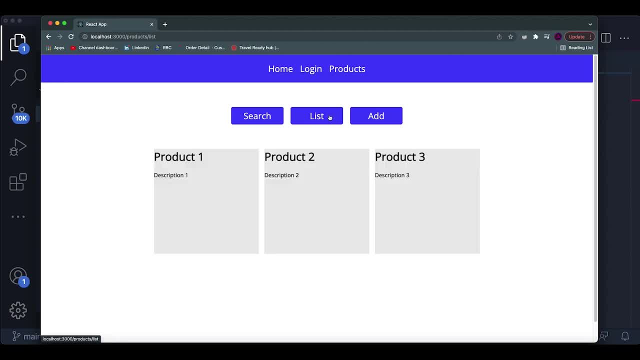 add product page if you want to. Also, if you want to click on one of the products, you can go to a specific page which only displays the information of that specific product. Those are various different examples of situations where you need to use nested routes because, in order to make 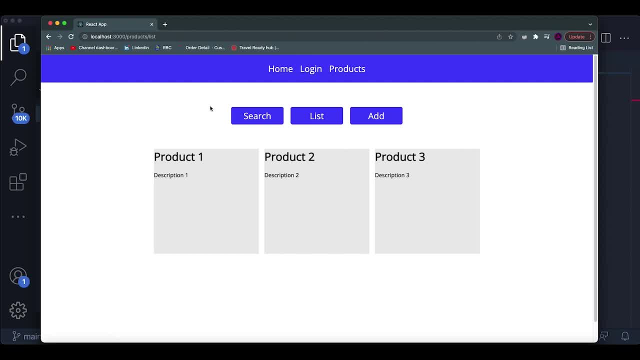 this work, you will have to implement it in a very concise way, in a very organized way, and React Router DOM provides you with that. So this is basically what we're going to be building. I'm just going to be focusing on the React Router aspect of it. I'm not going to be building the CSS and the 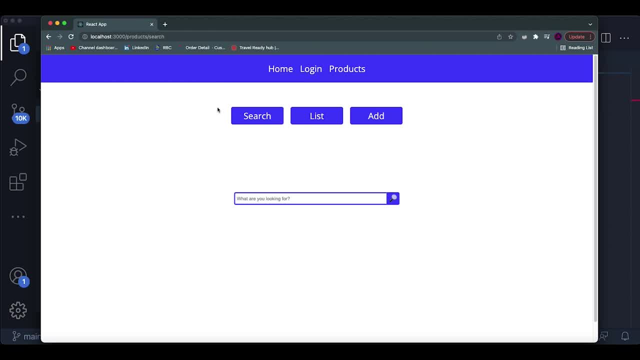 whole like HTML for this. This is already done, But I'm going to use this as an example in order to explain it to you guys. So, with that in mind, if you guys could leave a like for this video, it would help push my videos to more people, and just. 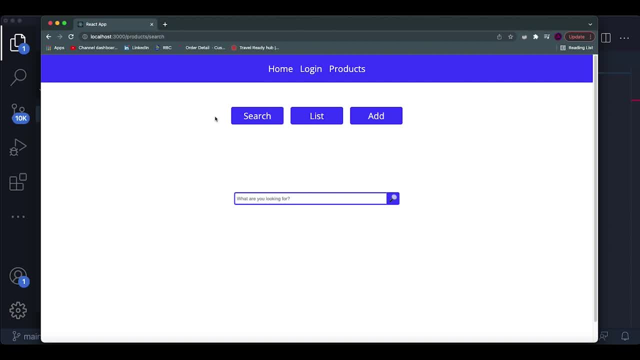 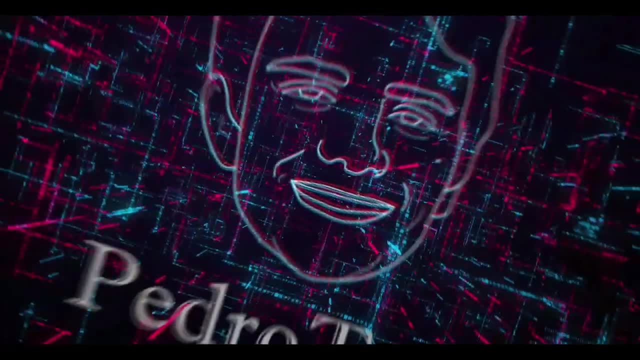 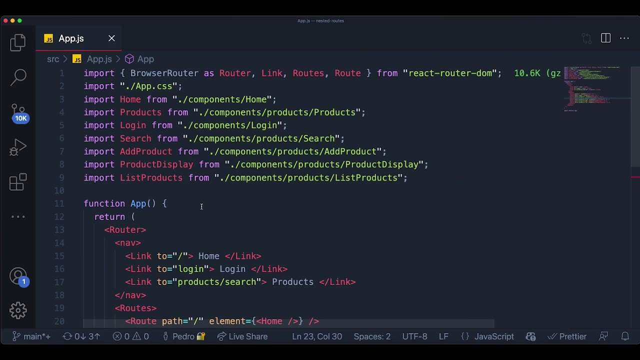 help support the channel overall. So, again, with that in mind, let's get into the tutorial. So now that I show you guys a demo, let's get into the tutorial. I have set up this little project over here, which, again, the code will be in the description. However, it is a very 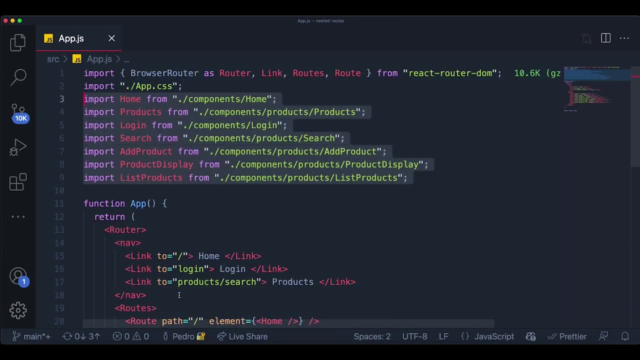 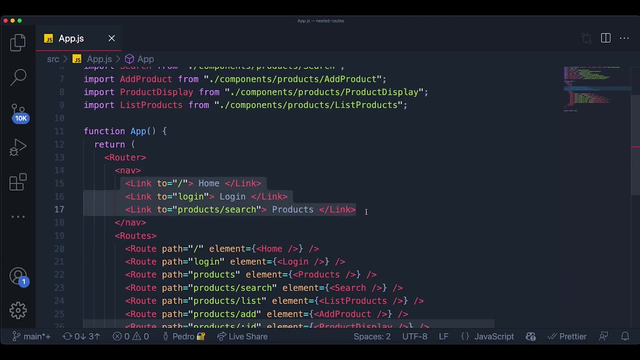 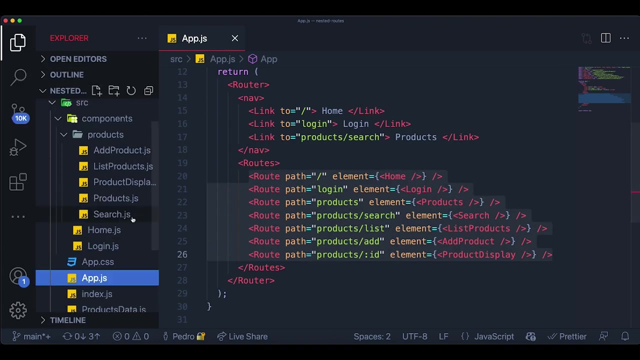 simple project. I know there's a lot of lines of code, but basically it's just creating the routes for the project, right? We have the navbar over here with the three links that we have in the navbar. Then we have all of our routes and all of their definitions. In this project we also have 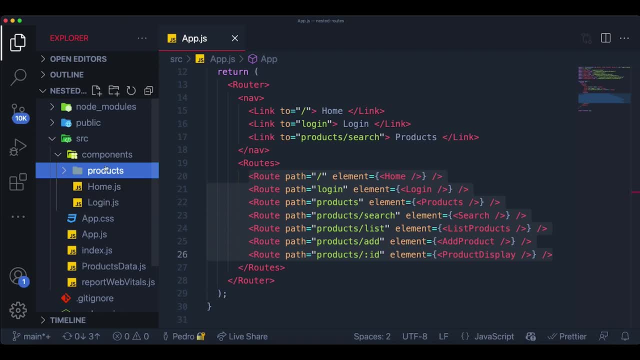 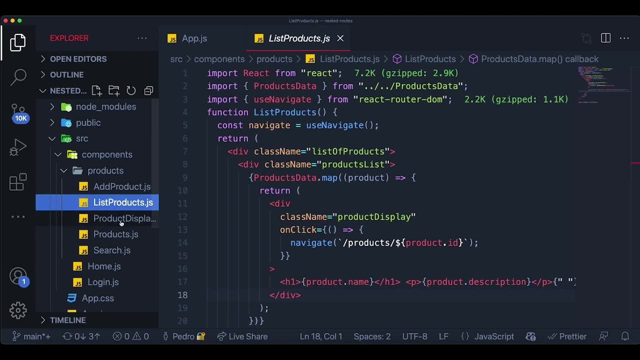 a folder for components: the home and the login component and also all of the different components that we have for the project. So let's get into the tutorial: The like, the products right, The list products, the product display, like page and everything. 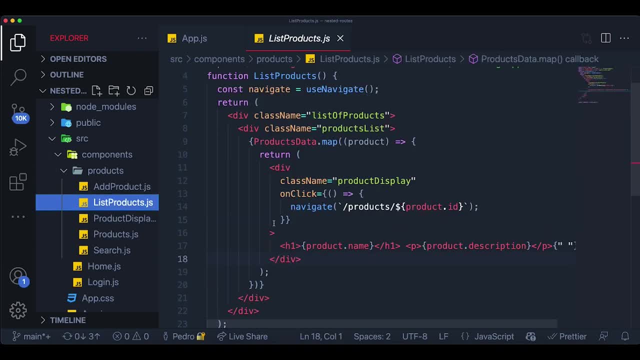 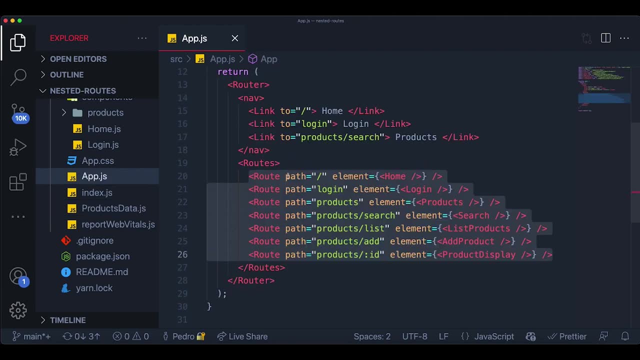 all of the logic for them. So everything inside of it, it doesn't really matter. I'm actually using fake data that I wrote over here for for the products. Again, you can just use them if you want to. that really doesn't matter for the point of the tutorial. What matters is the fact that if 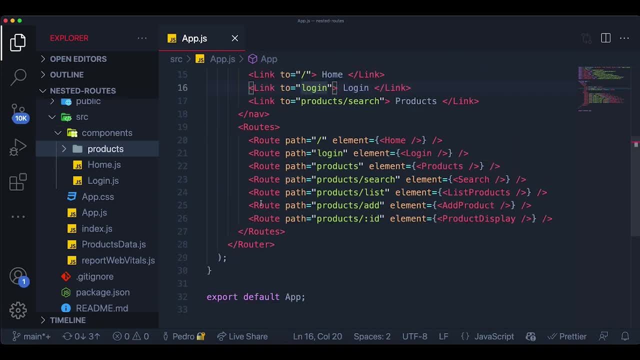 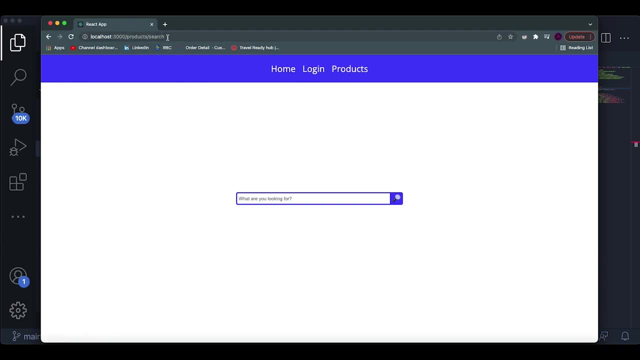 we go over here to our routes definition. you can see that if we wanted to like define the routes like we had over here, where you go to products, then you go to product slash search, then product slash um list, like all of those things. you can see it's already looking weird. it's already looking different from what it was before. 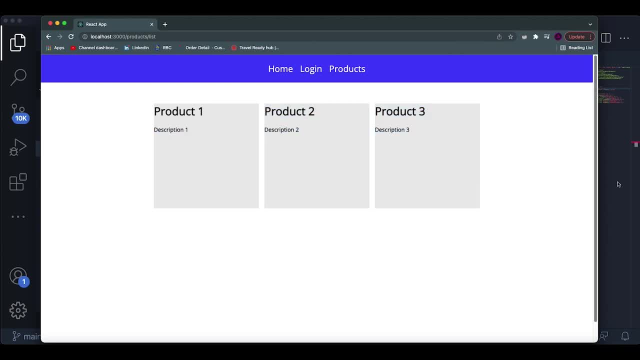 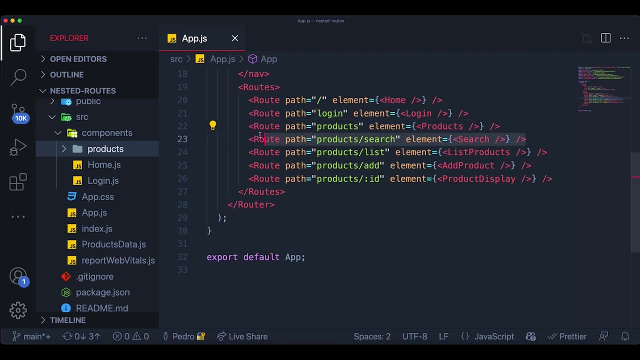 because we- i removed the implementation of nested routes in this project. so if we wanted to do something like this, we would have to define a different um route for each of the different specific routes that we want. so, like um for the product slash search would have to create a. 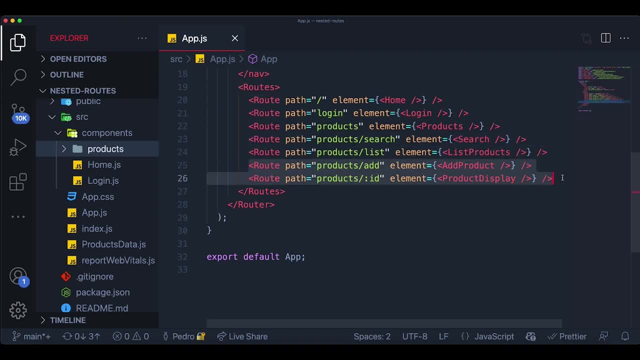 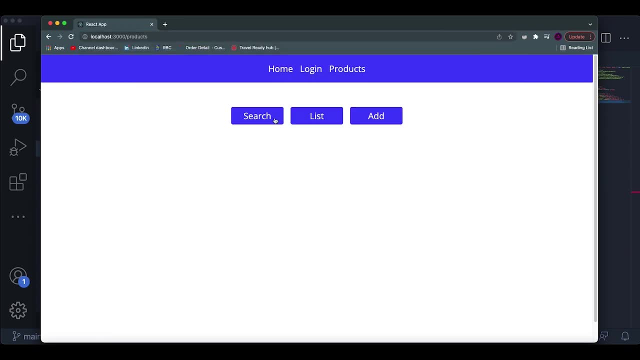 separate route for this, then one for this, then one for this and also um the, the navigation menu that we have in the products page, like the slash products page, this one over here. it doesn't exist on the other ones, it only exists on this one, which is kind of weird because, uh, we won't just have it. 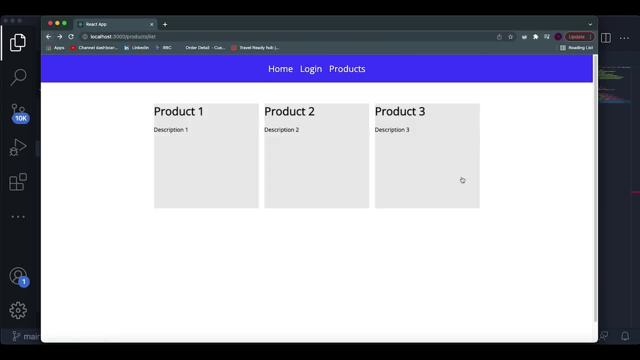 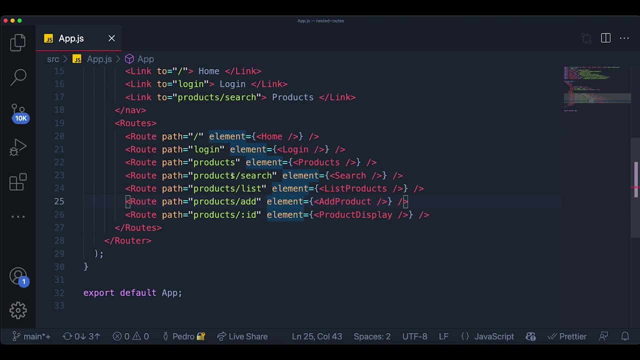 in every single one of the pages. um, so how exactly would we fix this and how exactly would we implement nested routes in this situation? well, the way we do this is very, very simple. we have this route, uh, like the main route for, for the nested routes, like system for, in this case, called the products route. 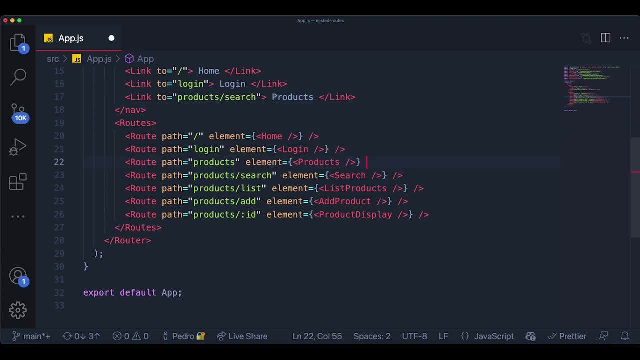 and in the products route. instead of self-closing like this, what we want to do is we want to actually um, enclose and wrap all of this around with this route component, then all of this um routes instead of here are now, uh, childs of the products route, and this means that we don't need 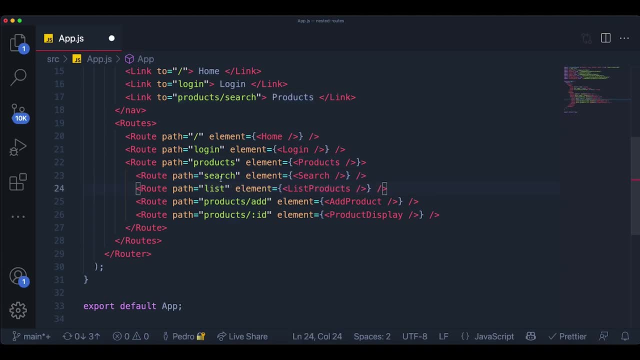 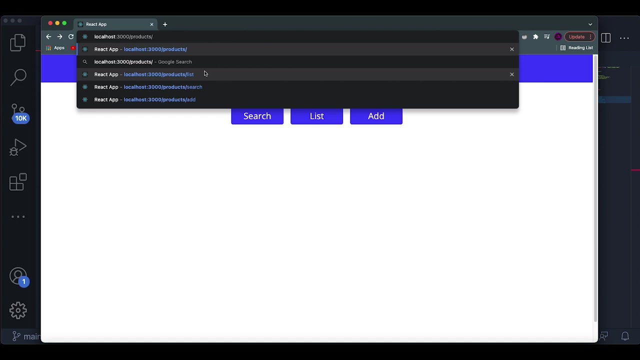 to put products anymore over here. you can just put the name of the route and it will automatically know um which route you're talking about. then, um, we have, and we now have all of this and you can see it still works perfectly. if i go to the list or to the um, let me see the search one: um, it seems. 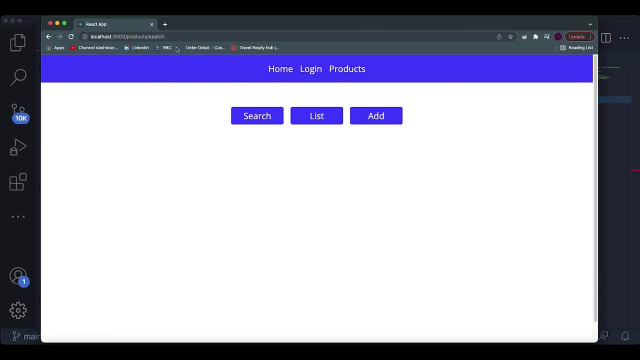 to work. right, it shows them the little navigation system that we have on the products, but it doesn't show anything specific to that page. right, if we go to the search one, it doesn't show the search bar, the list one doesn't show the list and the add one doesn't show the add um add product. 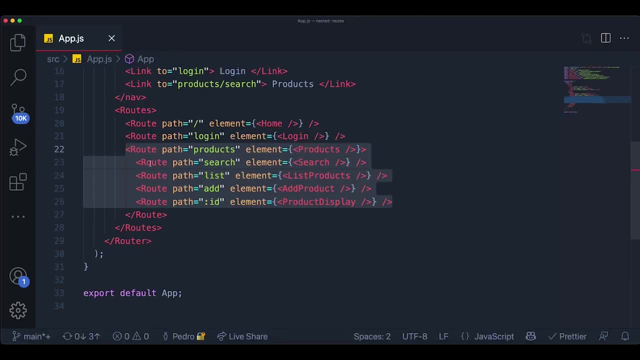 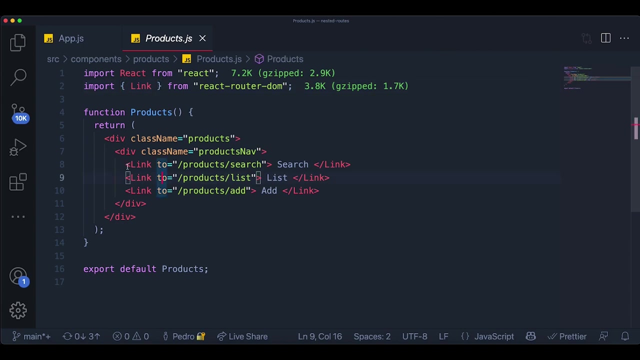 um thing right. the reason for that is because if you want to display a specific thing for each of the routes, so a specific component for each of the routes, you need to go to the main component, which is the products one um over here, and what you do is you add some sort of um common uh. 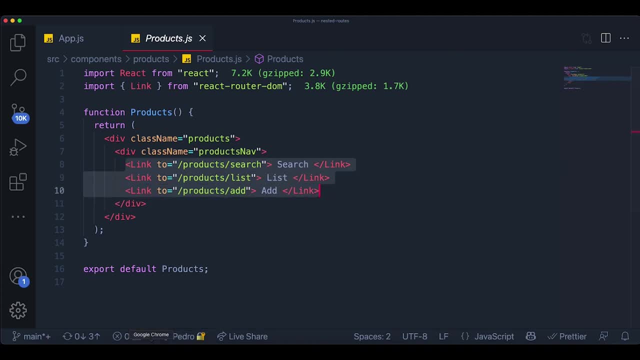 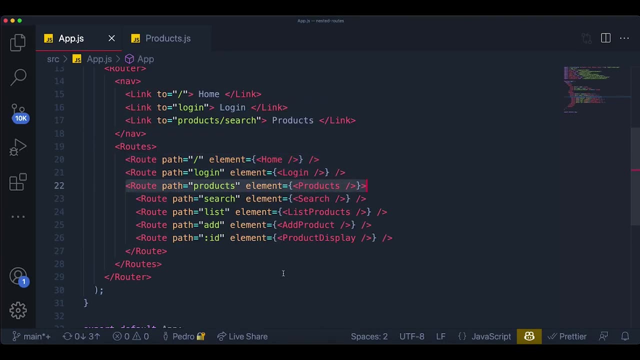 functionality or common ui for all the pages and in this case it is the little navigation here at the top or routes. right we have the login, the home and the products route, and in the products route we have a specific ui that we want to display for all of the different. 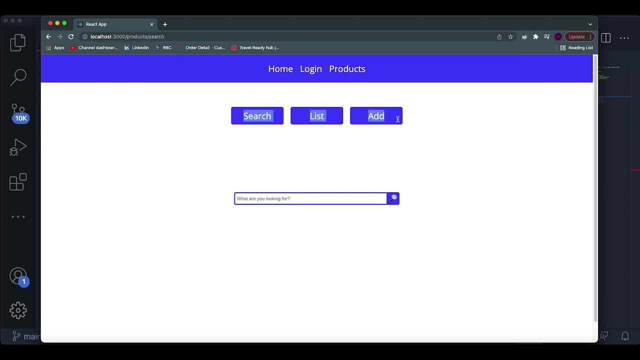 products routes. so in the search one, we still want to see this thing over here. for the list one, we also want to see this, and even if we go to a specific one, like a specific product, we also want to see all of this over here. the only thing that is changing in the page is whatever is below. 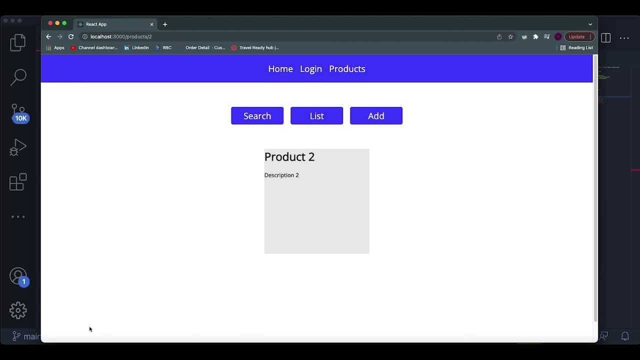 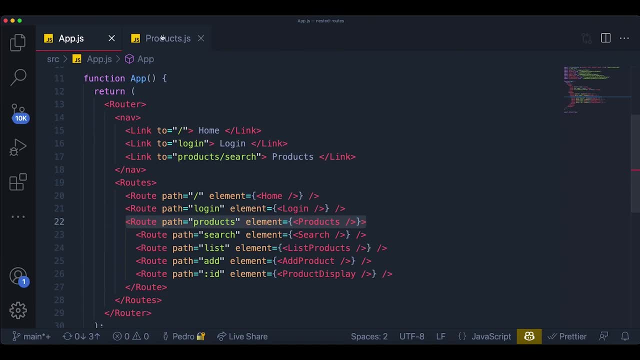 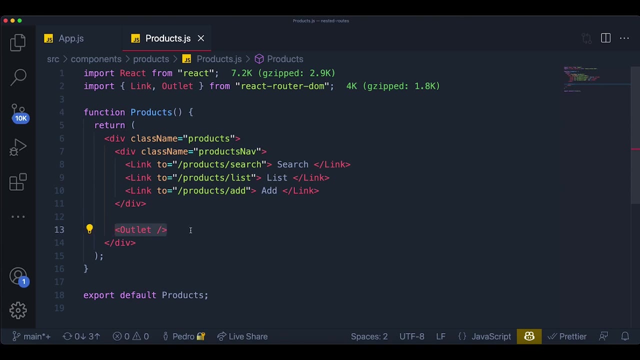 that right, this thing over here, and this is exactly what the outlet component is. the outlet component will replace wherever you put it in the in your code. so we put it right below the nav bar, just so that the network continues in the page, but the outlet um, but whatever is below it changes um and it will. 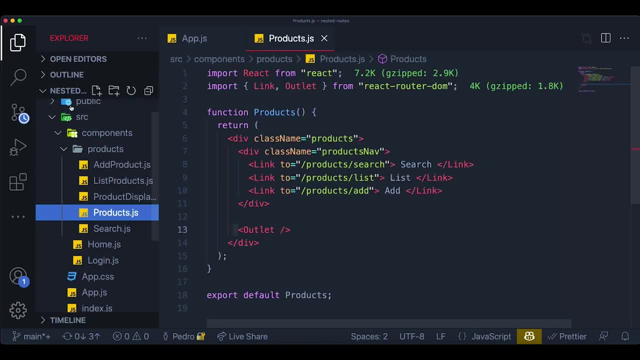 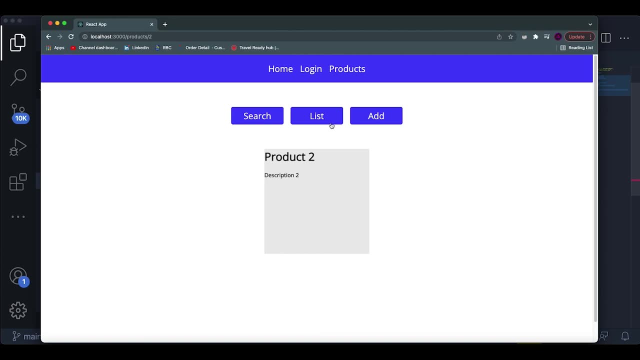 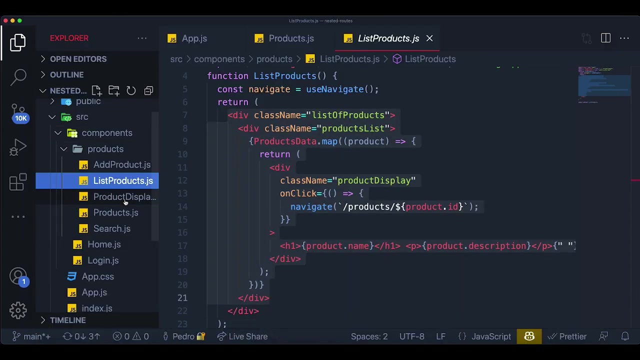 be replaced which whichever um component we defined over here. so in the list of products the outlet component will be replaced with this if we are in the um list routes. so we just keep replacing what that component with the other components that we defined based on the routes. 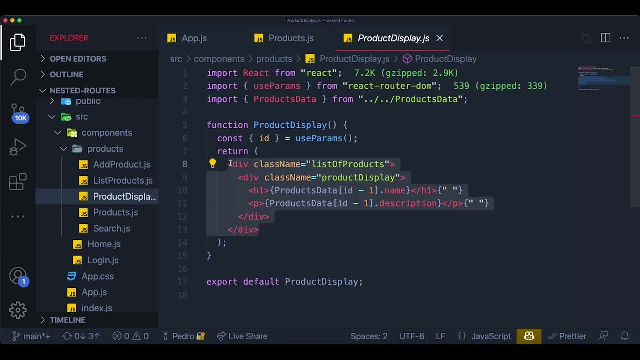 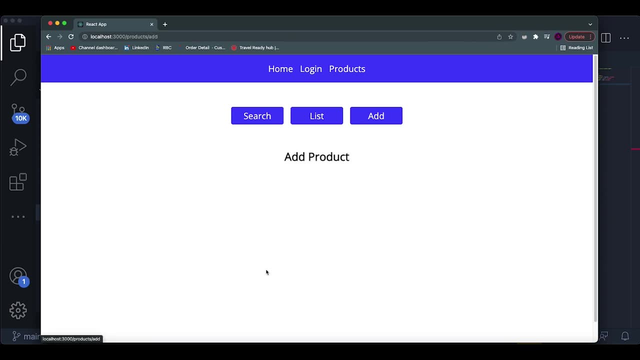 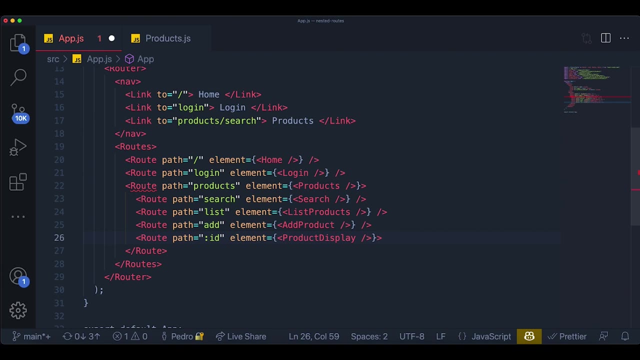 of the products. so if that's a bit confusing, don't worry, i would literally just play around with it. but, as you can see, um now everything works perfectly. um, you can even nest more and more um routes inside of other routes. for example, i have this id route over here which basically just displays the like one. 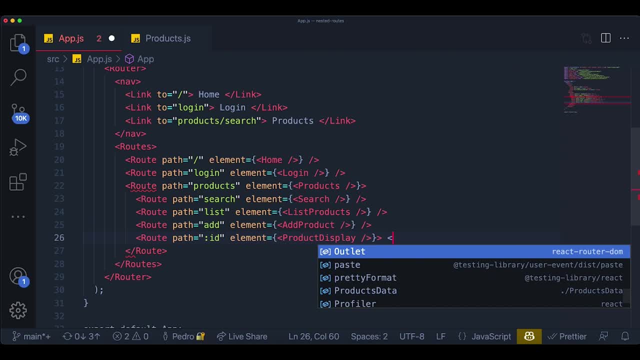 individual route. um, that when we click on it, right. so if i actually made this into another route, i could add more routes inside of here. um, and using the outlet would be the same thing, right, i would. i would just put the outlet and change whatever i want. now i don't want to do this. um, this was just 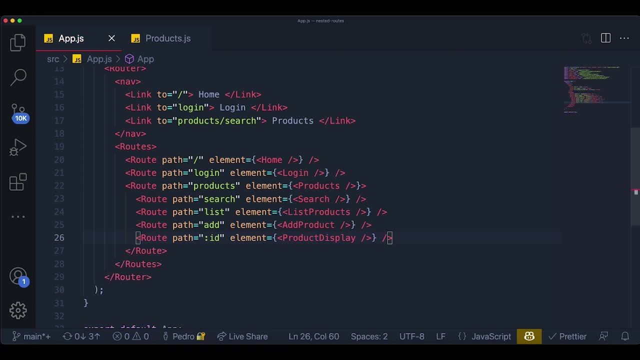 an example, but it's just to point out all the different cool stuff that you can do with this. now, this is something that isn't that complicated, um, but a lot of people have difficulties with it. in the beginning i certainly did, especially with the changes with react router, dom version 6.. 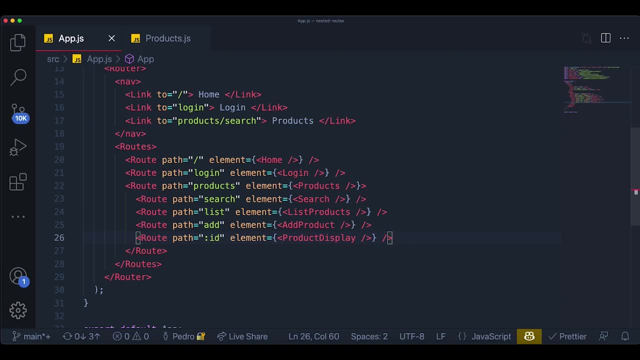 however, as i mentioned, i would play around with it and if you need more help and understand better react router dom, i do have a really, really nice video where i go over everything you need to know. that is actually important. i escape all the unnecessary stuff, um only the things you will. 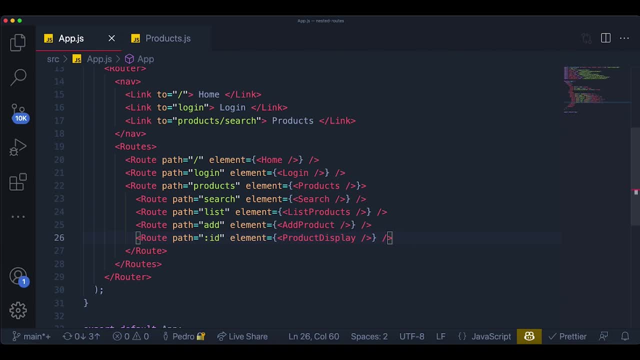 always use um and with react or dom, and i explain everything: um. so if you want to check out, i'm going to um tag it over here at the top and also put a link to it in the description. so this is a pretty short video. however, i really wanted to make this video just because a lot of you guys 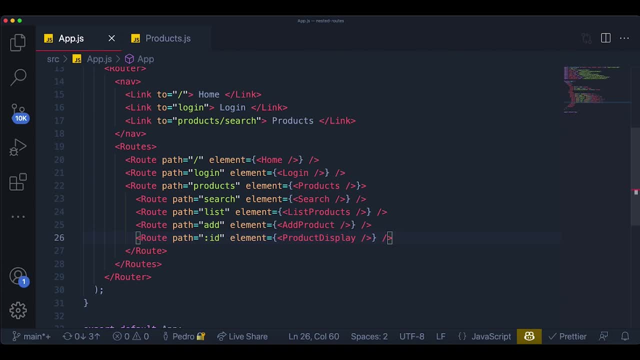 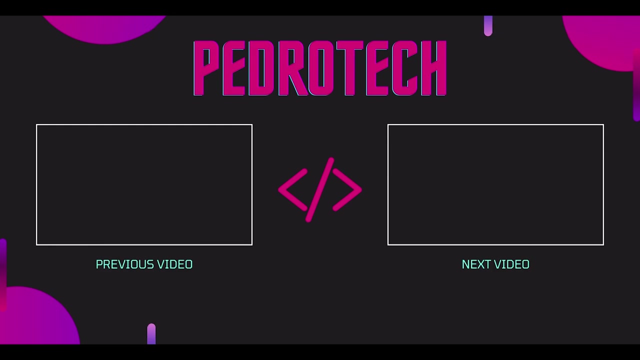 requested and if you enjoyed it, please leave a like down below and comment what you want to see next and subscribe if you want to support the channel. with that in mind, i really appreciate you guys watching this video and i see you guys next time. so 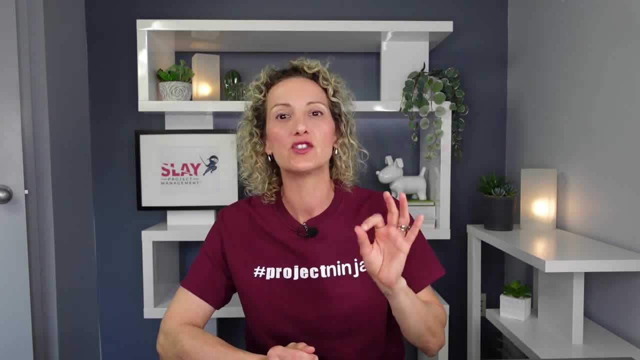 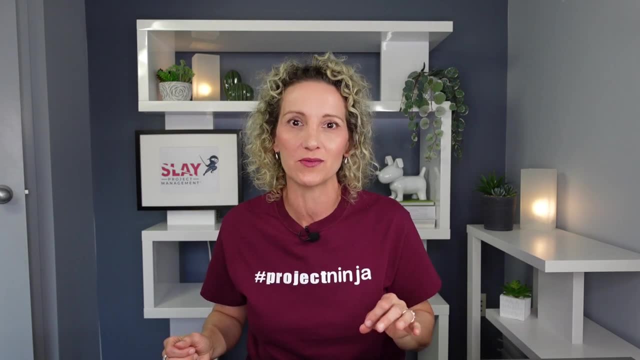 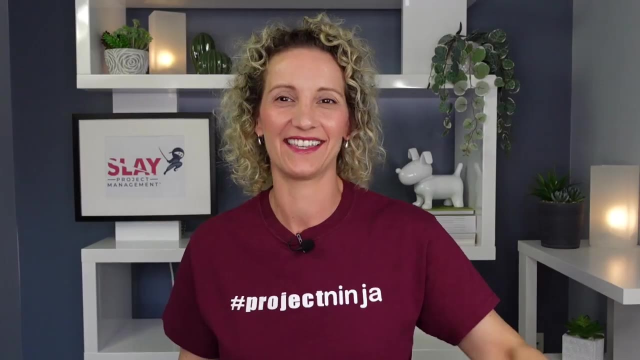 Your project communication plan is the blueprint to success for any project. They cite that most projects fail because they have a really poor communication plan or none at all, And in this video I'm going to share with you how to create an excellent project communication plan And if